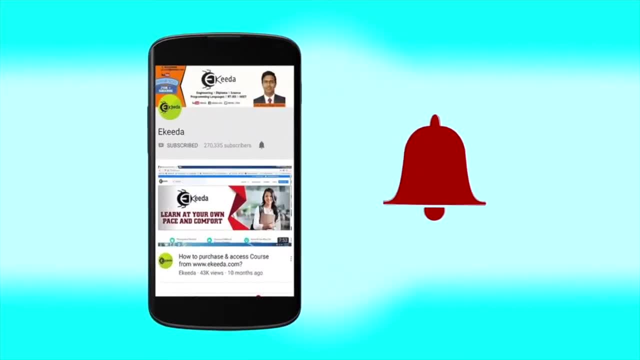 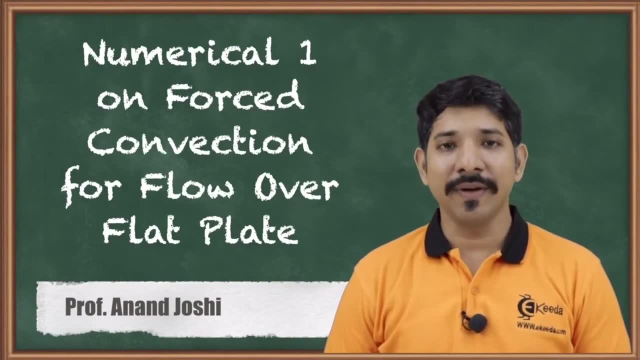 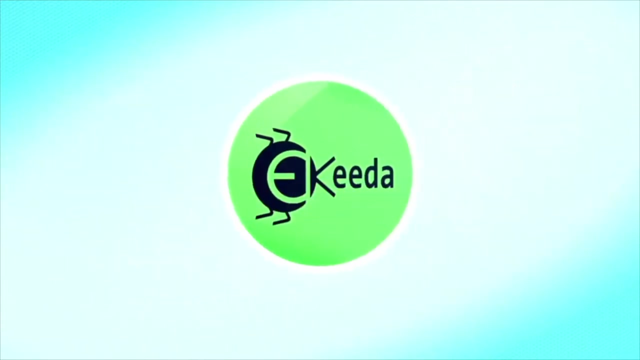 Hello friends, we have seen that in the analysis of force convection over a flat plate there are various core relationships that can be used. Now let us solve a problem based on that. to understand it fully, Let us read a problem. This is a problem on force convection. 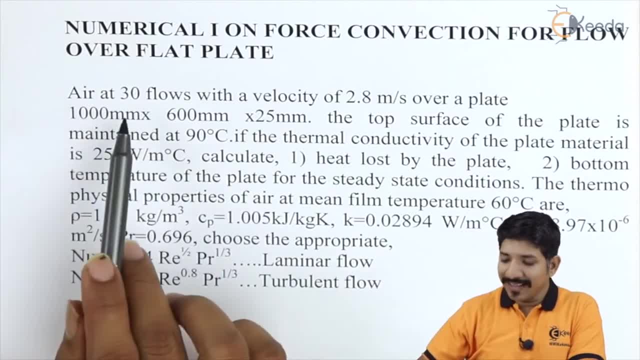 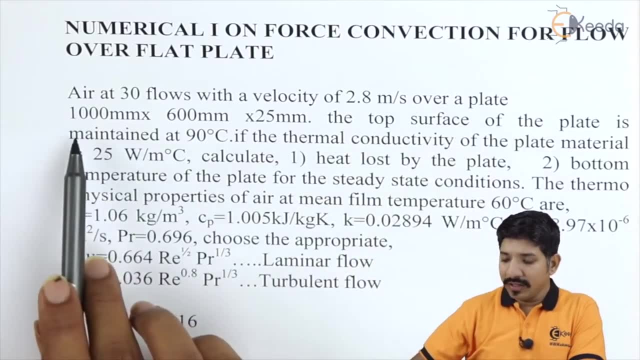 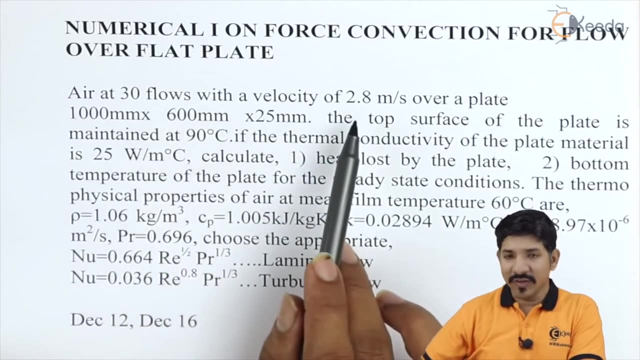 for a flow over a flat plate. The problem says air at 30 degrees Celsius flows with a velocity of 2.8 meter per second over a plate of 1000 mm by 60 mm by 25 mm. So they have given the temperature of the air, velocity of the air and dimensions of the plate. The 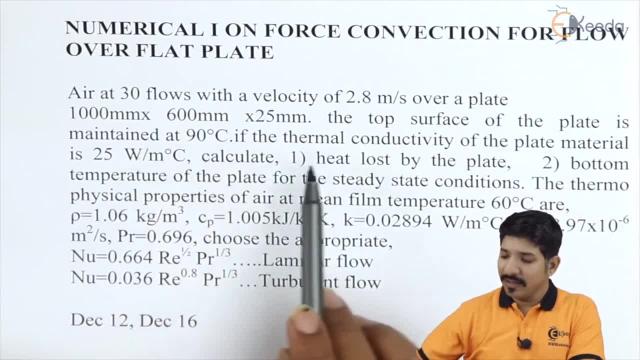 top surface of the plate is maintained at 90 degrees Celsius. If the thermal conductivity of the plate material is 25 watt per meter degree Celsius, calculate the heat loss by the plate. the bottom temperature of the plate for the steady state condition, the thermophysical. 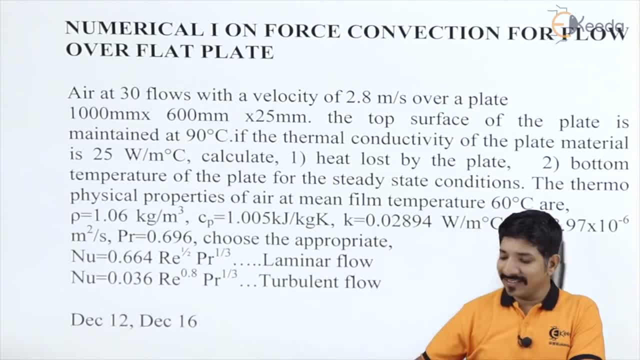 property of the air at the mean temperature 60 degrees Celsius, are given as: density is given 1.06.. kg per meter cube CP is given 1.005 kilojoules per kg kelvin. Small k, that is thermal conductivity, is given as 0.02894 watt per meter degree Celsius and kinematic viscosity, that is mu. 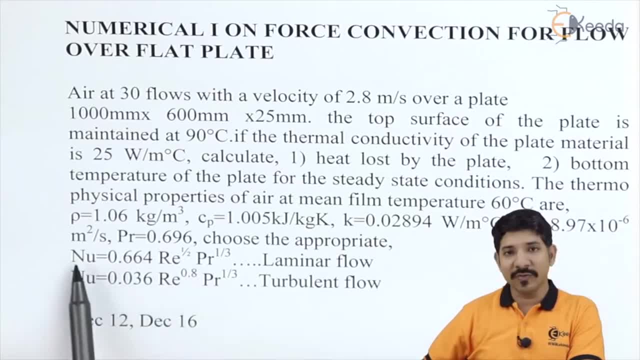 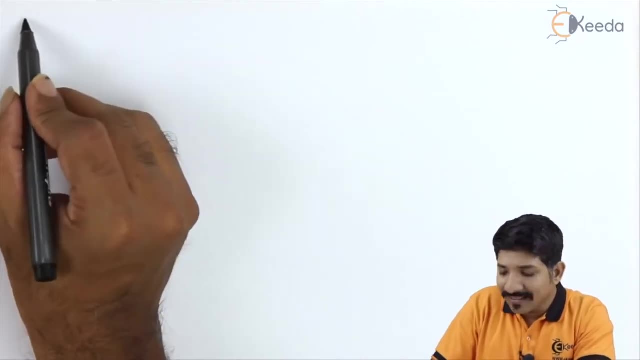 is given 18.97 into 10 to the minus 6 meter square per second. Prandtl number is given as 0.696 and they have given us two appropriate core relationships, One for laminar force flow and the other for the turbulent flow. Now let us draw the diagram for this case. 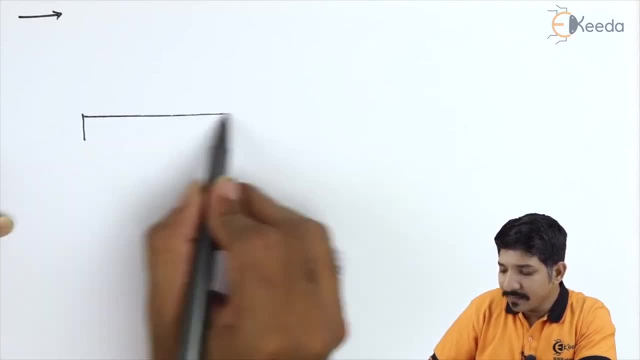 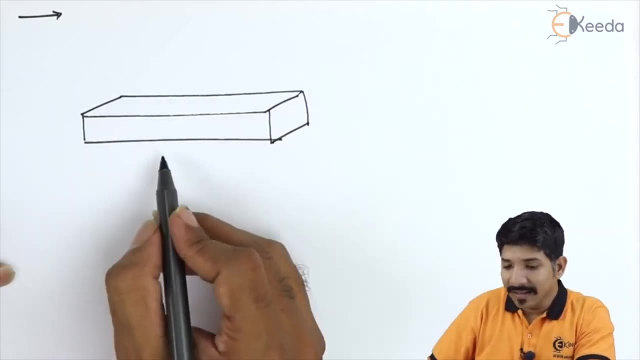 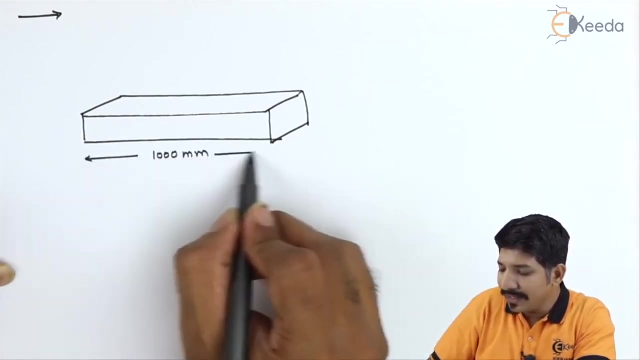 First thing is we will try to draw a plate diagram. So for plate, they have given the length as 1000 mm. So this is my length of the plate. Then they have given this width as 600 mm. So this is my length of the plate. Then they have given this width as 600 mm. 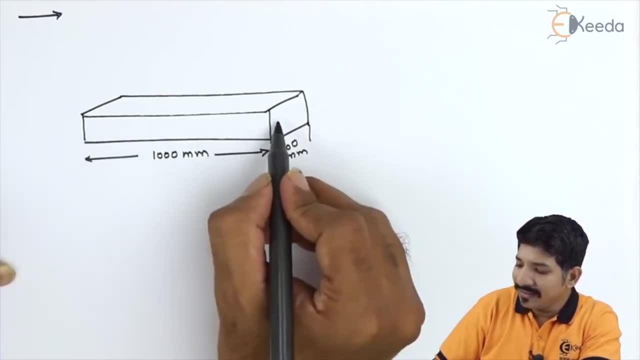 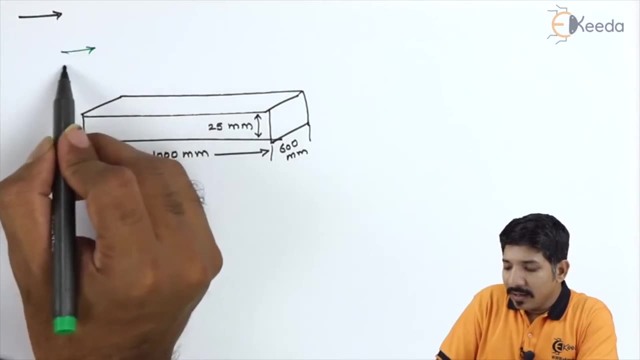 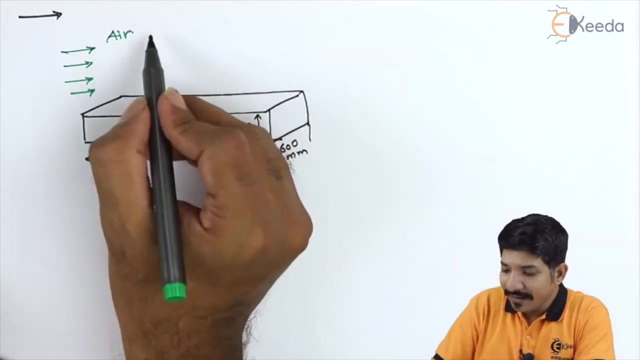 And the thickness of the plate is 25 mm, They have given that the air flows above it. And for air they have given us the temperature. So let us call this T infinity, Then the velocity is given. Let us call this U. Let us say the heat transfer coefficient is 0.5.. So this: 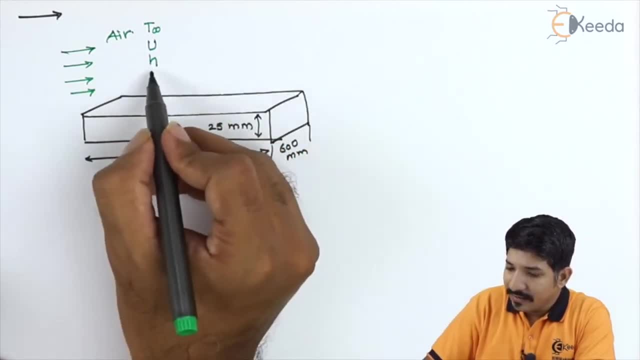 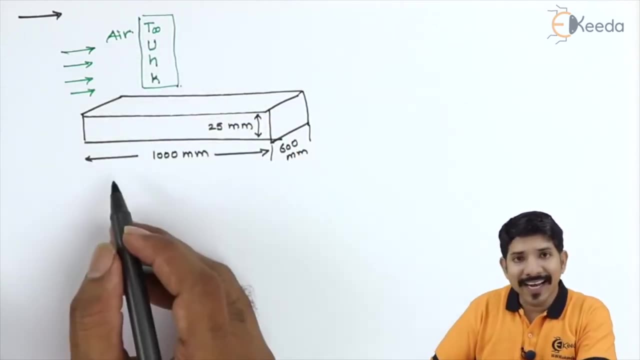 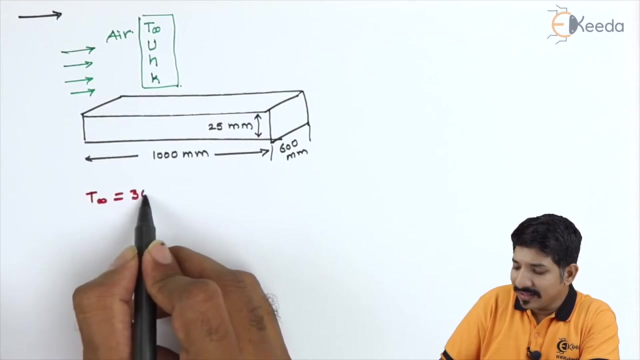 coefficient is H And thermal conductivity is K. Now let us write down the data that they have given. They have given us that the air temperature is 30 degree Celsius. Velocity- that is the capital U, is 2.8 meter per second. Then the dimensions are given. Then we have 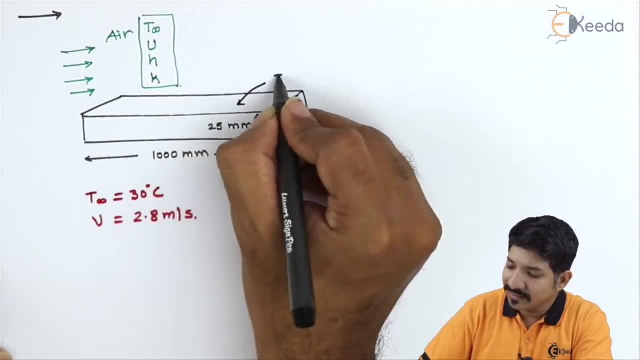 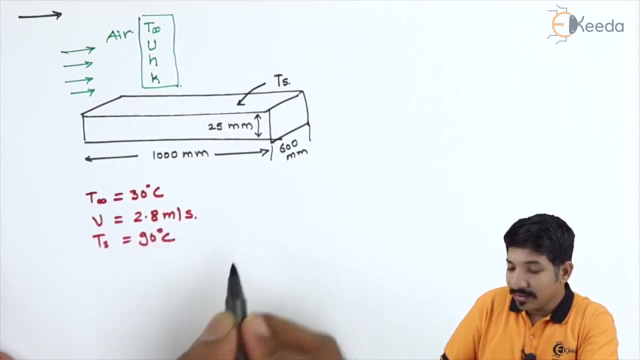 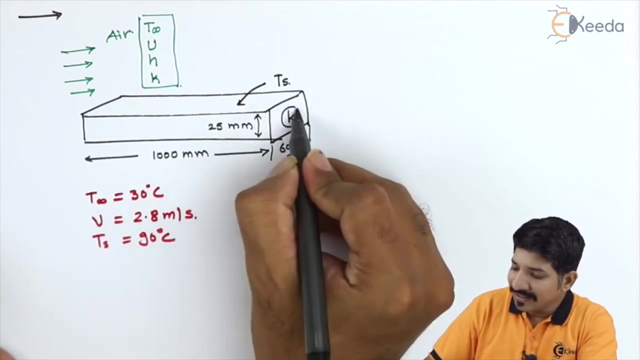 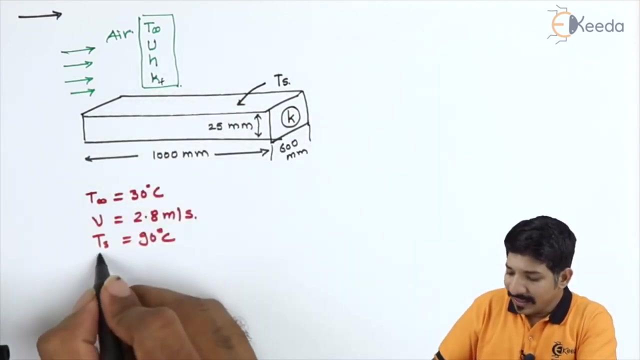 given the temperature. Let us call this as the surface temperature- T s. They have given T s as 90 degree Celsius With: if K is the thermal conductivity of, let's say, the plate and K f is the thermal conductivity of the fluid, Then they have given the value of K. 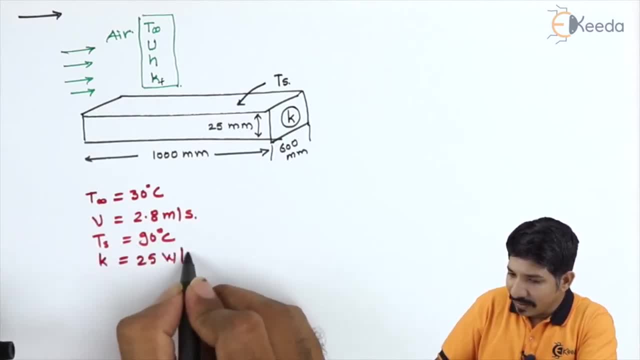 as 25 Watt per second. So this is the thermal conductivity of the plate. Then they have given the value of K as 25 Watt per second. Then they have given the value of K as 25 Watt per second. Then they have given the value of T? s. Now what do we have? Let's say the temperature. 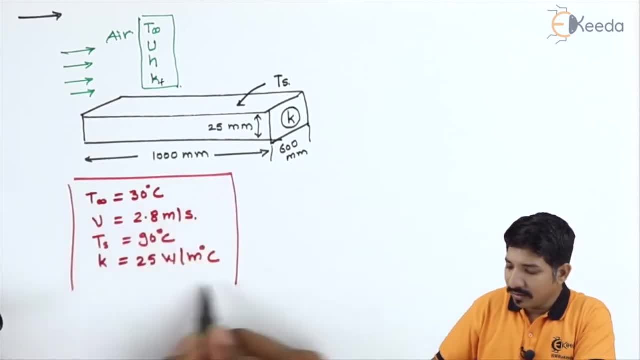 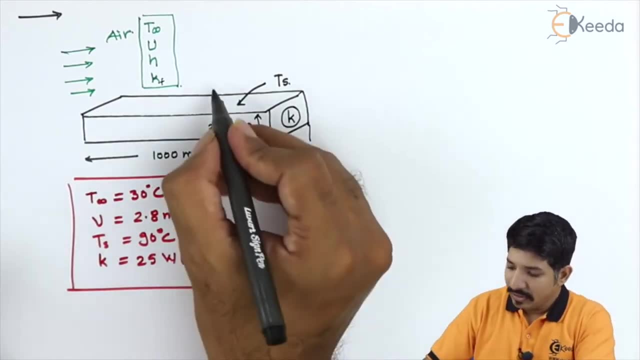 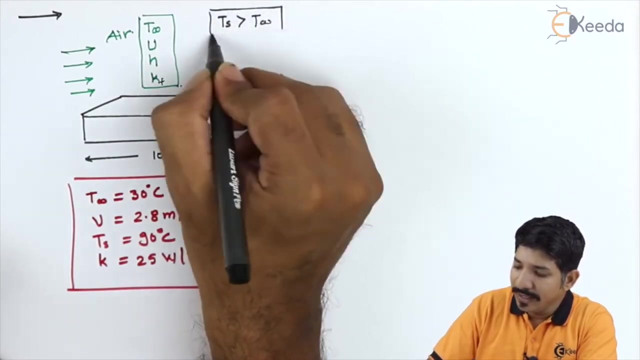 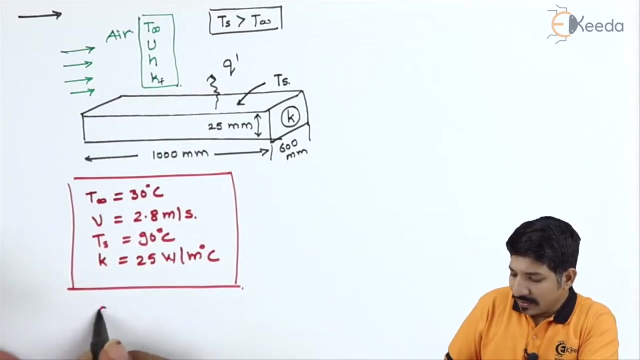 is 50 degree Celsius. Now, these many things they have given, and they are asking us to find out the heat loss by the plate. Since I can write down that T s is greater than T, infinity, The heat will be lost by the plate. Let's say the heat loss is given as Q dash. So they are asking us to find out. 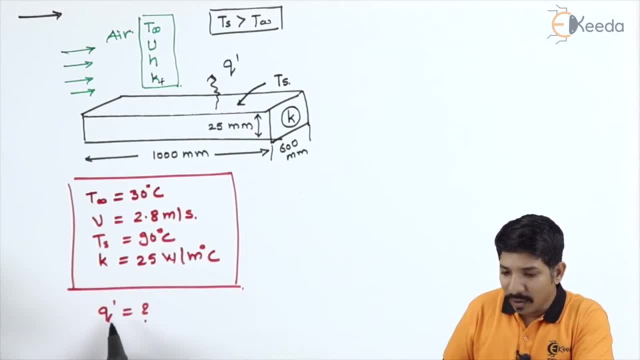 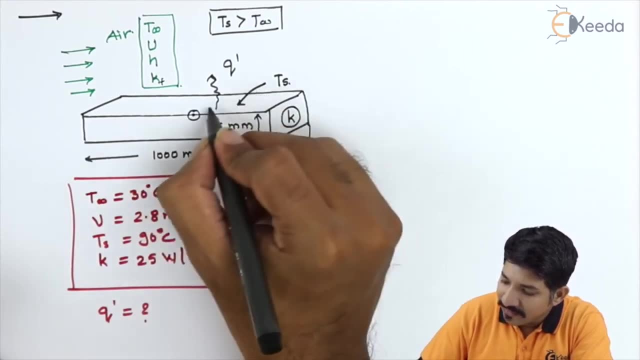 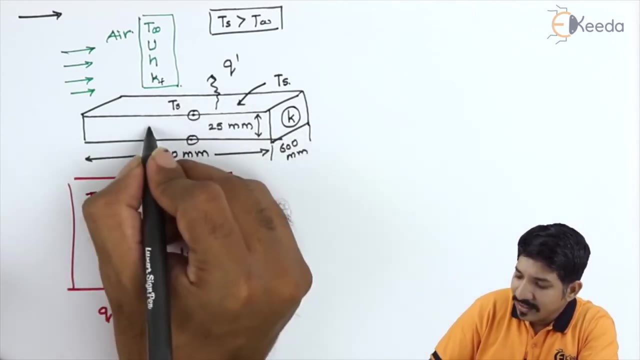 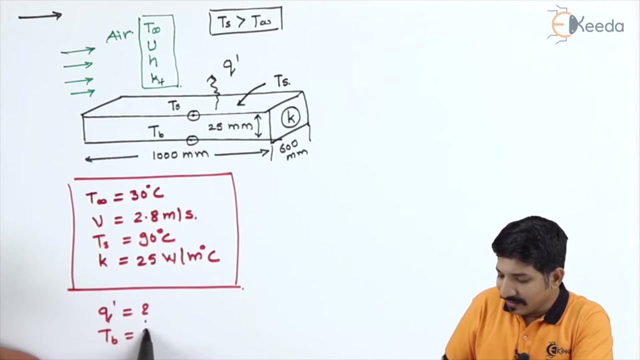 the value of q, dash. and then the second thing is bottom temperature of the plate. so let's say: if this is the value of ts, that is the surface temperature. they are asking us what is the bottom temperature? let us call the bottom temperature as tb. so what is tb is what they are asking. 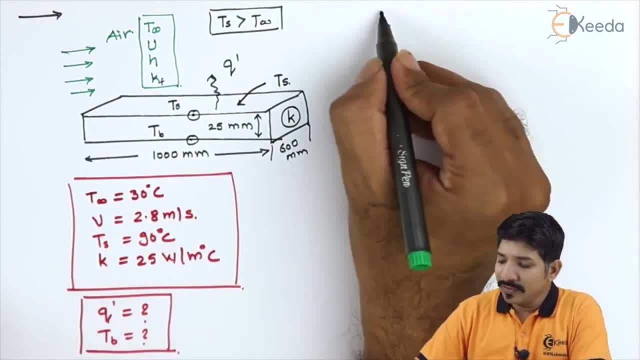 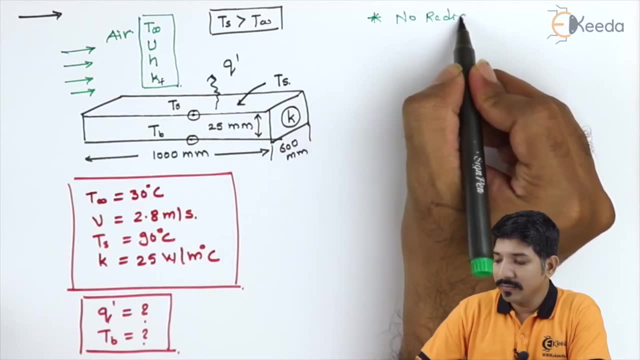 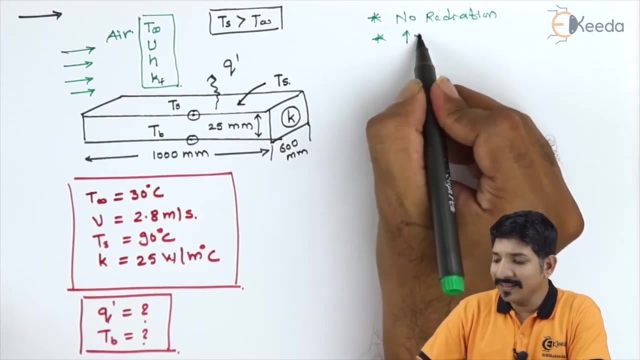 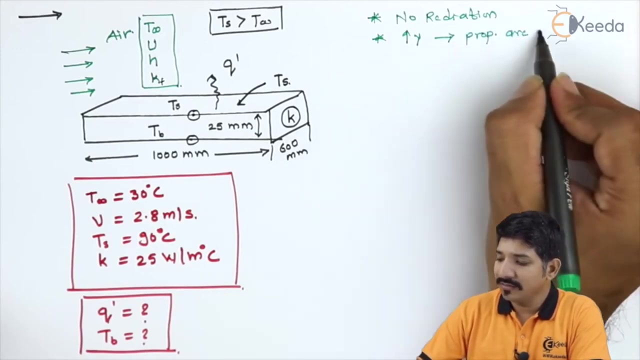 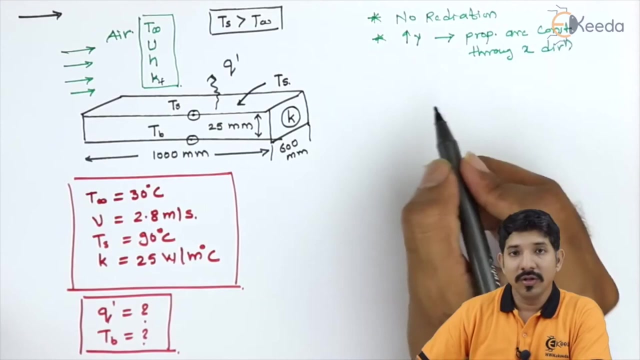 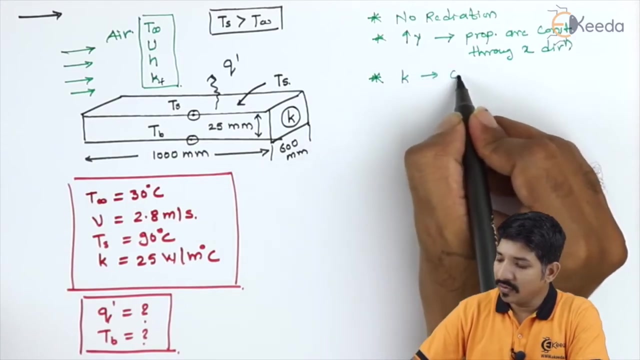 now let us start solving this problem, but before that we need to assume few things. what are those? such as no radiation involved, then the heat flow only takes place in y direction, so the value of or the properties are constant. through x direction, then the thermal conductivity is a constant parameter. 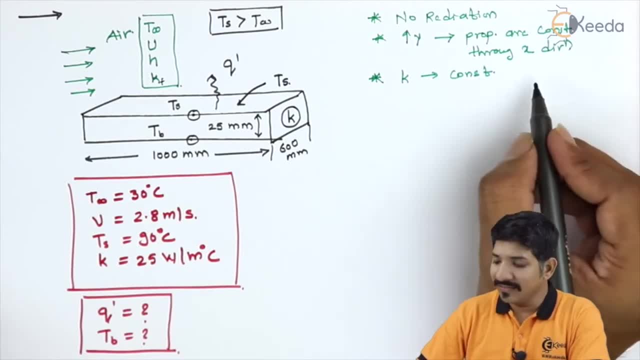 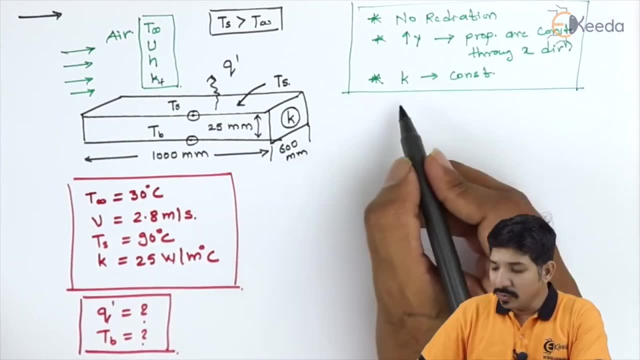 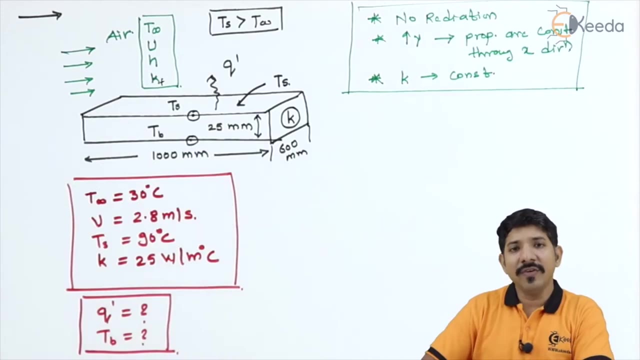 so these are the few of the important assumptions that we can follow. now for the solution, now how to go forward with this solution. so for this, first thing that we need to identify is if the flow is a laminar flow or a turbulent flow. so how to do that? we know that it can be done with the help of reynold number. 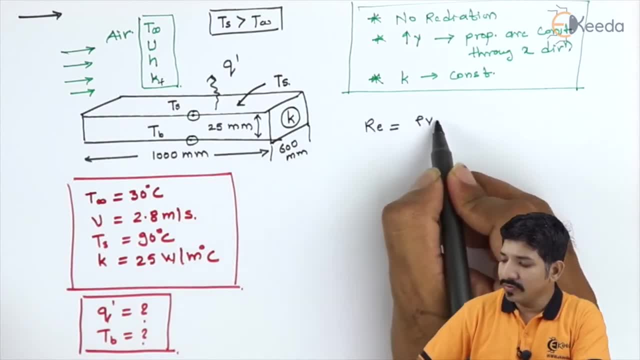 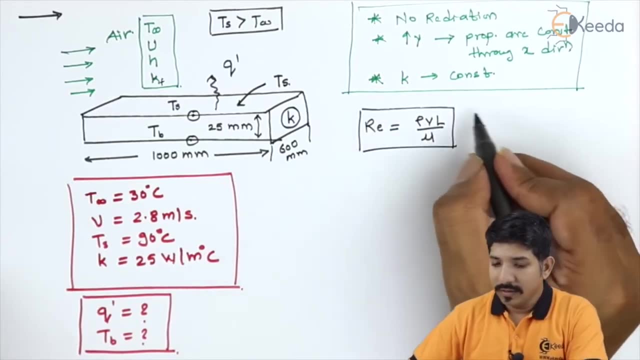 reynold number is given as rho v l upon mu. now, in this case they have not given us the dynamic viscosity, so we can write down mu upon density, that is the kinematic viscosity. henceforth the equation becomes the capital u into length upon the kinematic viscosity. so let us put the number 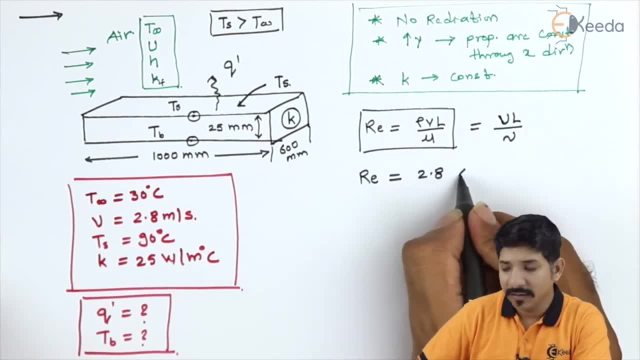 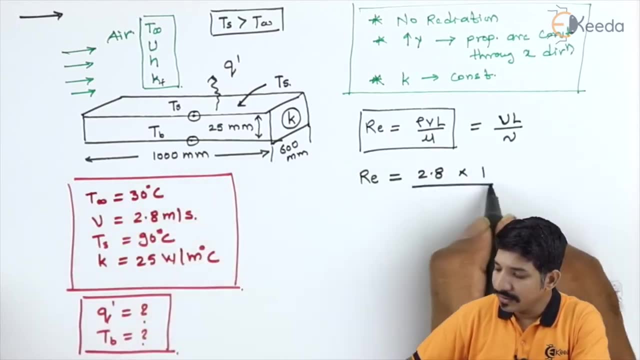 velocity is given as 2.8 meter per second. the length, the total length is 1000 meter, so that makes it one meter. divided by the kinematic viscosity, which is given as eighteen point nine, seven into ten raise to minus six. now they have given us the properties. 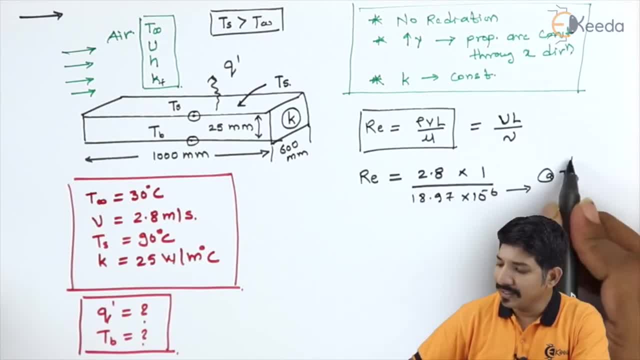 at the mean temperature. so the mean temperature in our case is obviously the temperature that you are given is 30 and 90, so my mean temperature will become 60. so at 60 degrees celsius. they have given us various properties, so those we are going to use. 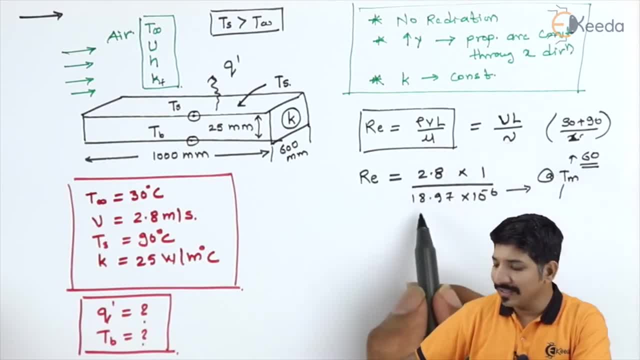 such as in case of dynamic viscosity. they have given this as 18.97 into 10 raised to minus 6. so if I solve this for the renal number, then we are getting the renal number as 1.47 into 10 raised to 5. 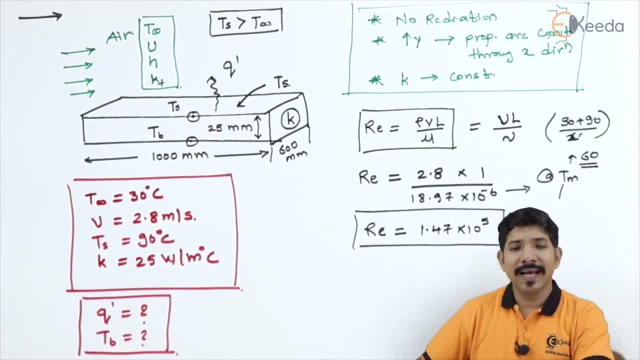 now we know that in case of a flow over a flat plate, if the renal number is less than 3 into 10 raised to 5, then the flow must be a laminar flow, since it is less than 3 into 10 raised to 5. 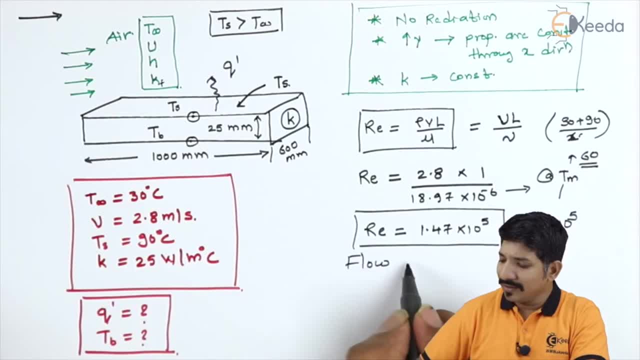 I can claim that the flow is a laminar flow. now for laminar flow. the relationship that they have given is 0.664, renal number raised to 1 by 2 and Prandtl number raised to 1 by 3. now we know the value of. 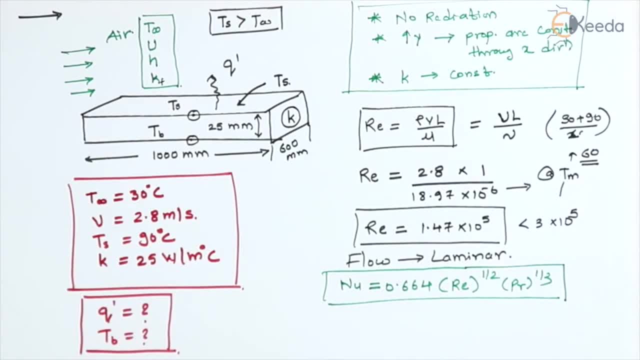 Prandtl number that they have given as 0.69 and the renal number we have already found out, so let us substitute the same number and find the nusselt number. so if I put the renal number as 1.47 into 10, raised to 5, and Prandtl number that they have given is 0.696, 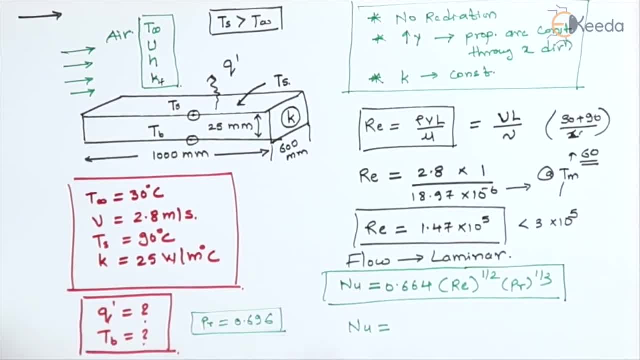 this is given, then the nusselt number that we are getting is. so, instead of finding nusselt number, we can straight away find the value of H itself. nusselt number is given as H, L upon K, where the value of L is nothing but, again, the length of the. 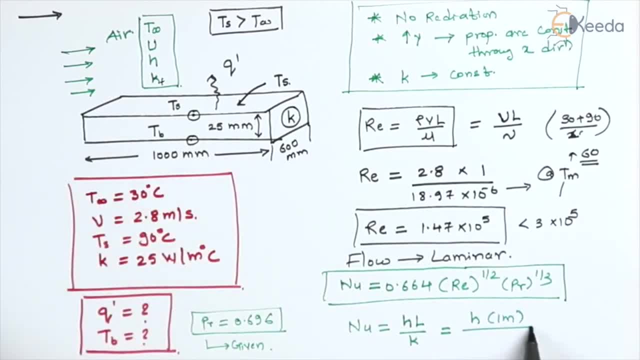 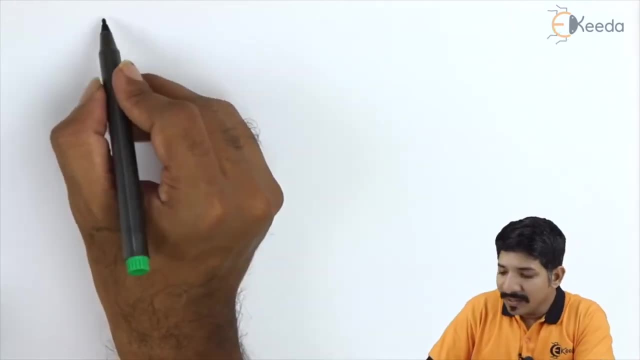 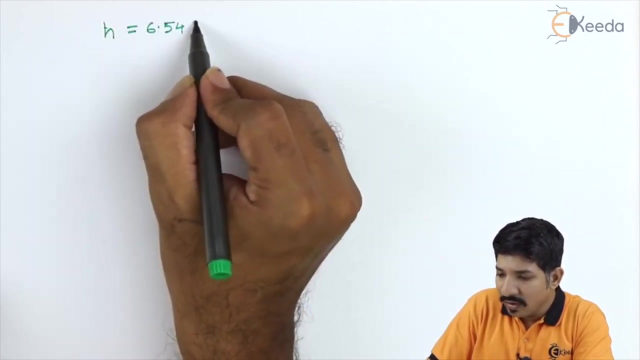 pipe that is 1 meter and the thermal conductivity that they have given is 0.02. we got the TH. now, if you solve this, we will get some Nusselt number. so if you solve the previous equation, then we can find the heat transfer coefficient as 6.54 Wad per meter. 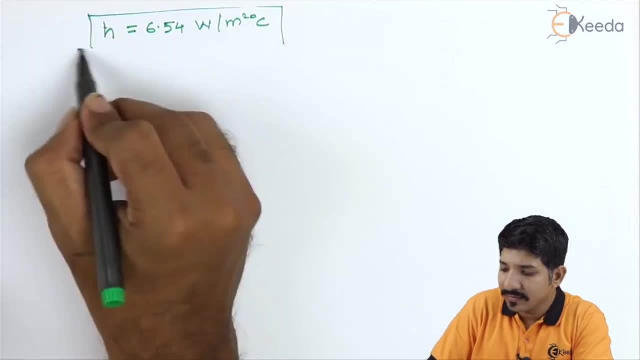 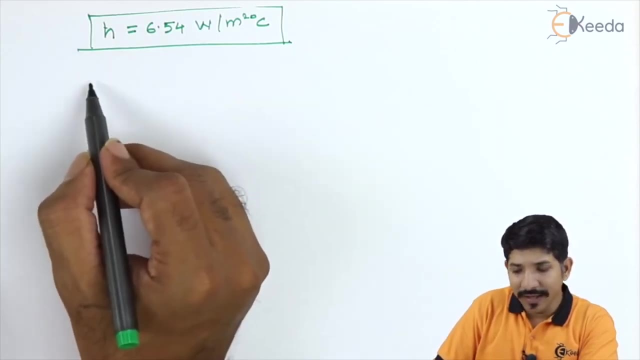 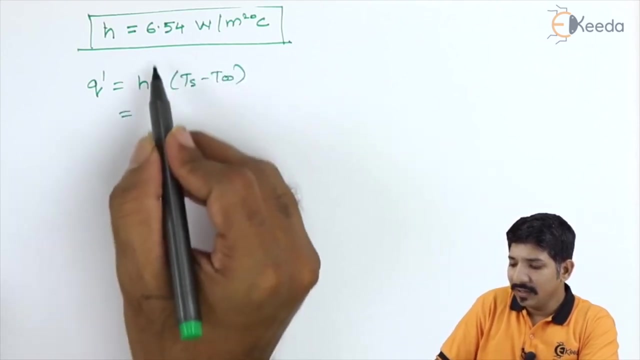 square degree Celsius. now this is the heat transfer coefficient that we have got. now we know that by Newton's law of cooling the value of Q' is given as Lbreq, H, A, T, S minus T, infinity. so the value of H is 6.54. the value of area is the surface area. 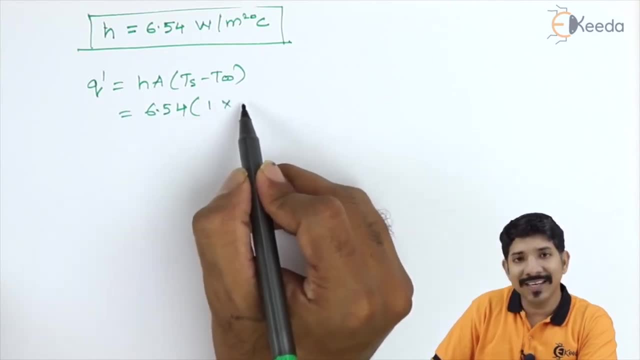 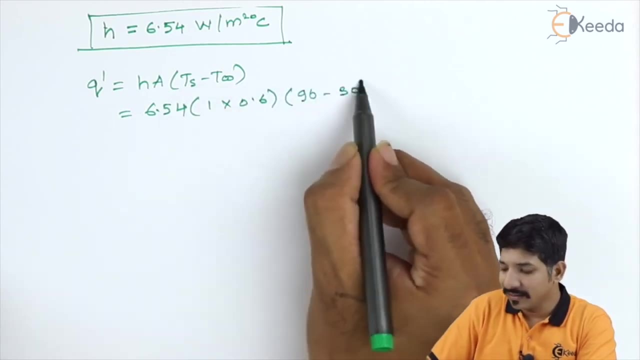 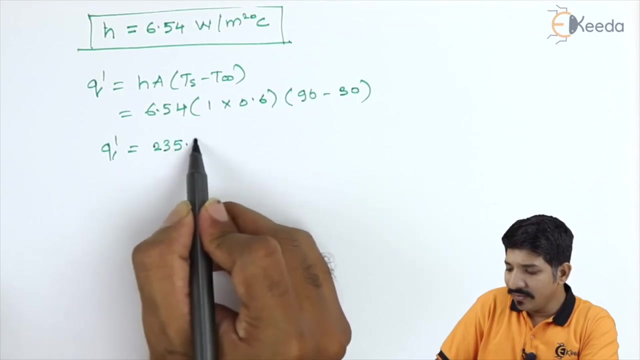 that is 1 meter by 600 mm, so that is 0.6, surface temperature is 90 and the air temperature is 30.. so with the help of this we can find the value of q dash that they are getting as 235.4 Watt. 235 Watt is the amount of heat that is liberated by the plate to the air. 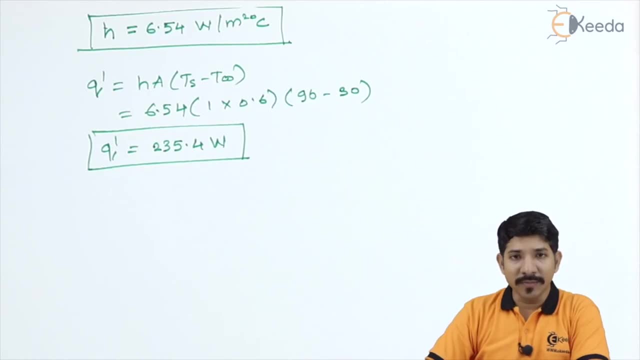 the second case, and they are asking us to find out the bottom temperature of the plate. now for that. we will assume that the same amount of heat that is converted to the air is also conducted through the plate, and we can use the Fourier's equation to find that. 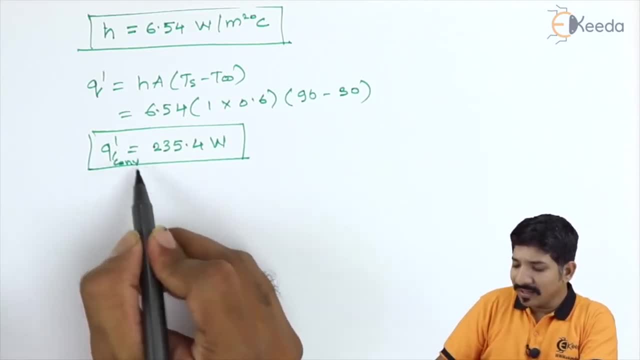 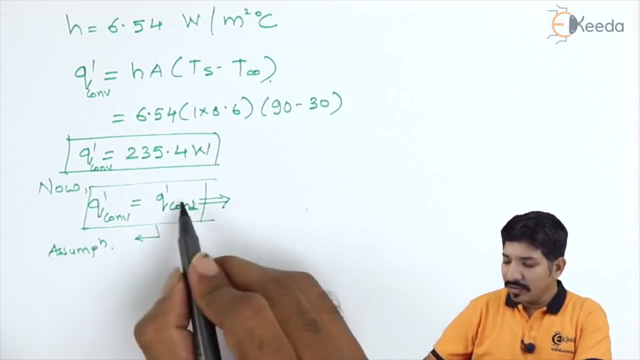 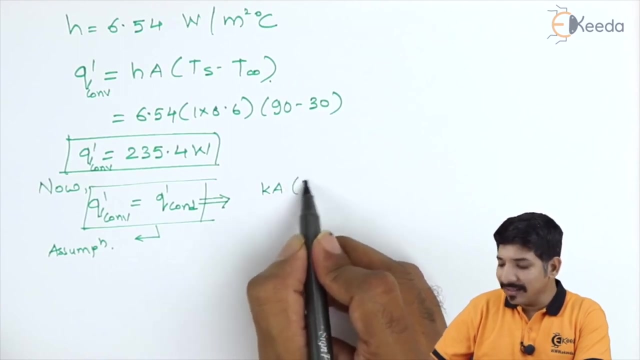 temperature. so let us do that. so now, this was the convicted air here. we are going to assume that the q dash of convection is same as q dash of conduction and by Fourier's law the q dash of conduction is written as K, A, delta T. now, in this case, my delta T is the surface temperature and bottom temperature. 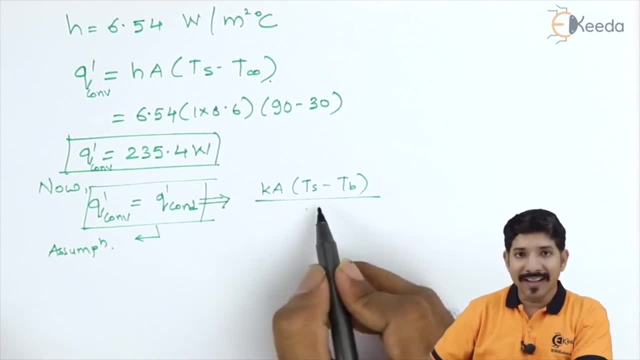 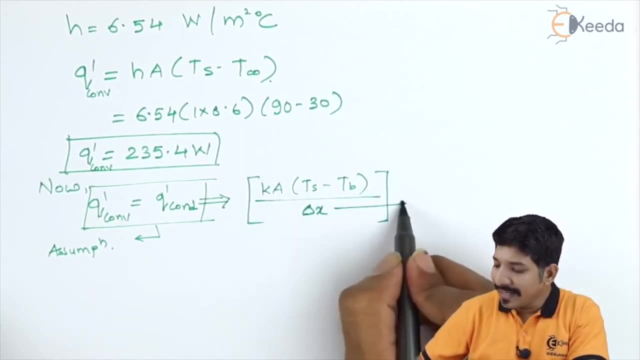 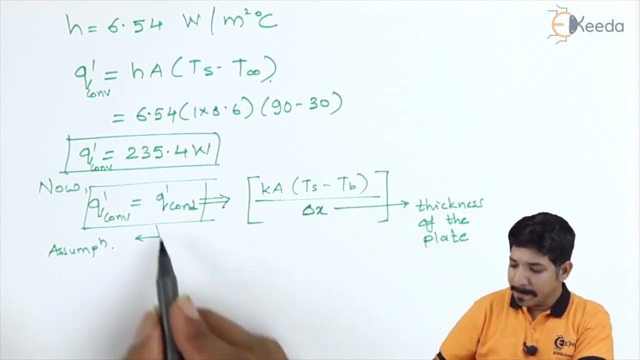 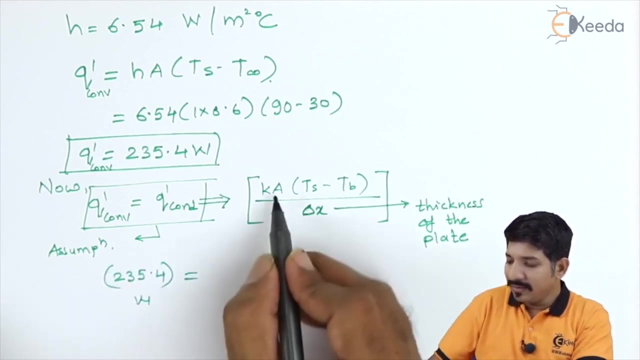 and here the length is nothing but delta x and the bottom is delta x. now here, my delta x is nothing but the thickness of the plate. now again here everything is known. we will simply substitute the numbers to get the unknown. the q dash is 235.4. this is what we assume is equal to K, the thermal conductor to the. 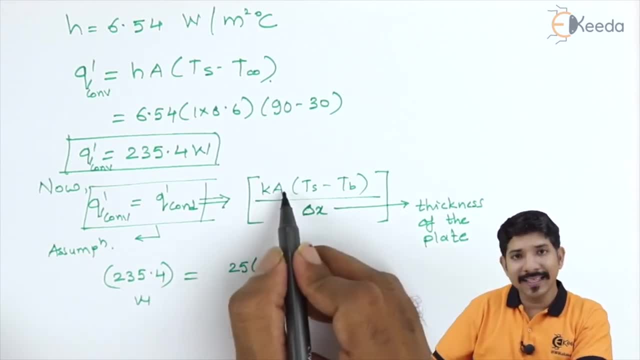 plate that we have given is 25. the area in this case is my surface area itself, so that is 1000 mm. that is 1 meter x 600 mm, that is 0.6 meter. surface temperature they have given is 90 and the bottom temperature is what is unknown. so we will. 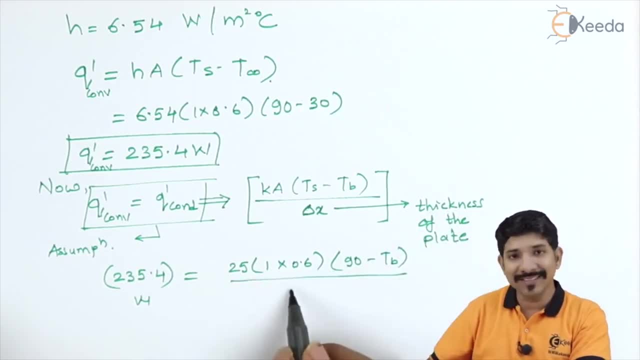 write this as tb itself divided by thickness. now, thickness is they have given as 25 mm. this is 25 into 10, raise to minus 3.. now, again in this equation, the only unknown that we are having is tb. so if you solve this, the value of tb that we are getting is 90.39 degree Celsius. now, as you. 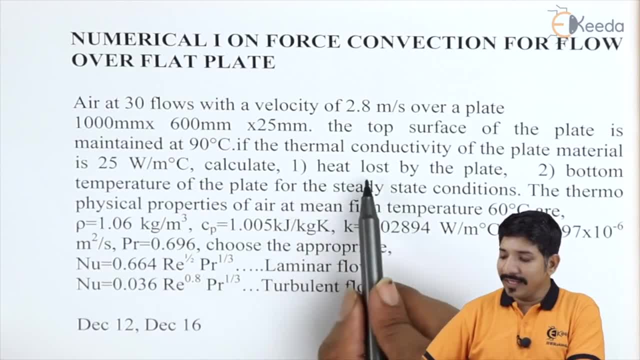 can see in this question. they ask us to find out the heat loss by the plate. so we got the heat loss around 235 watt and they ask us to find the bottom temperature of the plate for steady state condition. now, this was the assumption that we have already considered, so that bottom 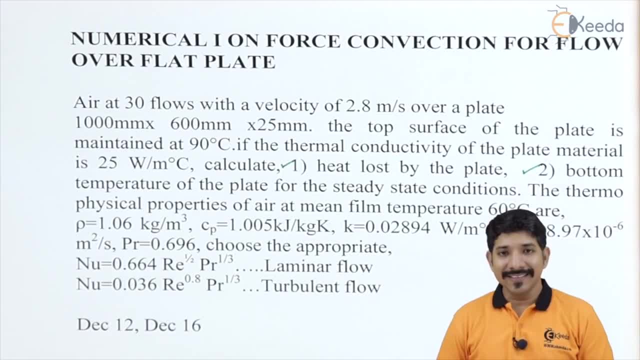 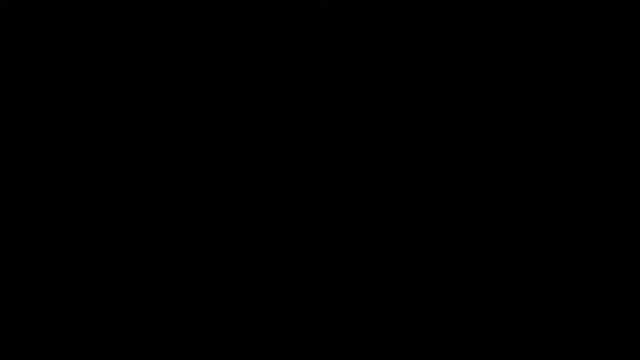 temperature that we got is 90.39 degree Celsius. that is it in this problem. thank you for watching this video. please stay tuned with eKIDA and subscribe to eKIDA. thank you you. 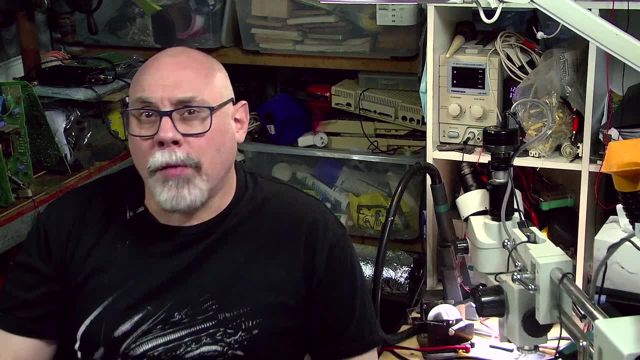 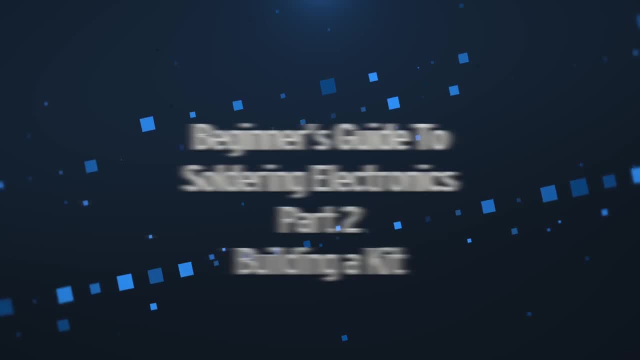 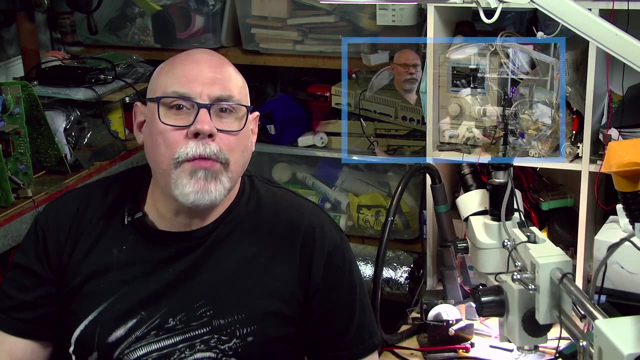 Hi there, my name's Bruce Rayne from Brankus Creations, and this is my Beginner's Guide to Soldering Electronics, Part 2.. Before we get started, I'd like to mention my Beginner's Guide to Soldering Electronics, Part 1.. 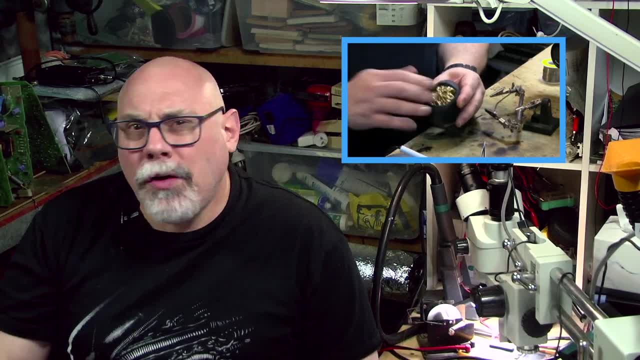 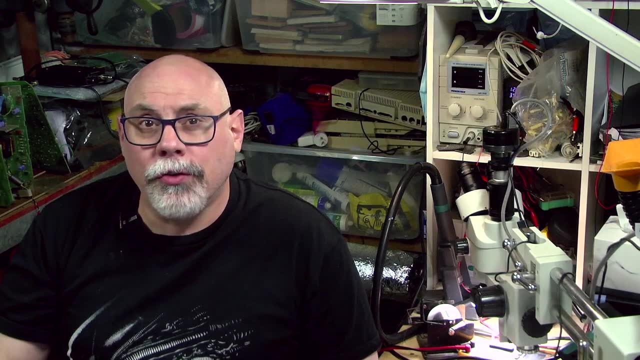 If you haven't seen it, I'd recommend taking a look. Although I don't do a whole lot of soldering, in the video I do explain a lot of important information that could help you get better soldering results. Kits are a fun way to get into electronics and practice your soldering skills. 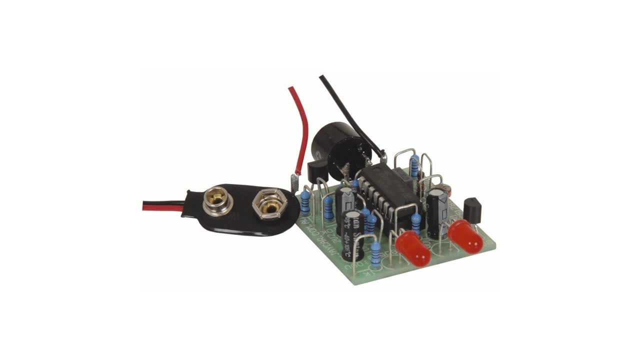 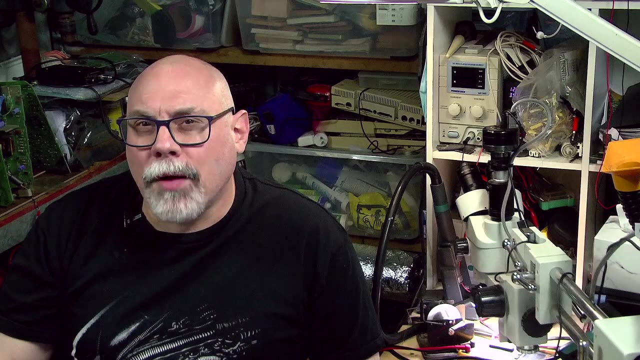 You can find kits for all skill levels, starting with a simple one like this that makes a noise like a cricket, all the way up to building a whole computer from scratch. I like to make kits with some sort of practical purpose, so I'll be doing this demonstration with a capacitor testing kit. 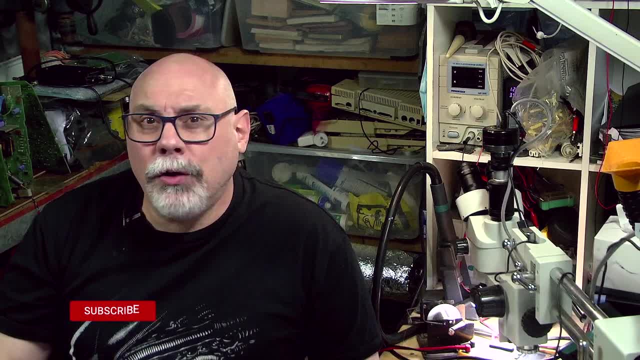 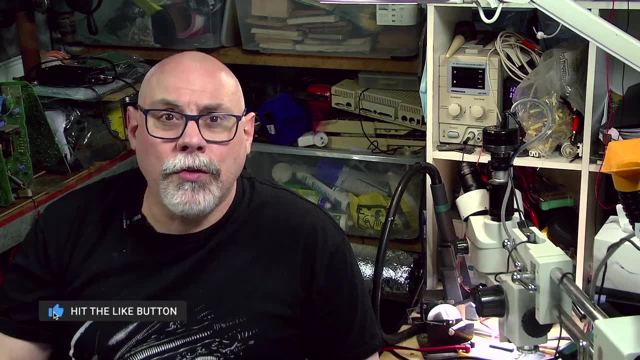 Once complete, I'll be able to use it to test capacitors. I've included some links in the description to places where you will find some great kits to buy. You'll also find links to all of the equipment I use, as well as some budget alternatives. 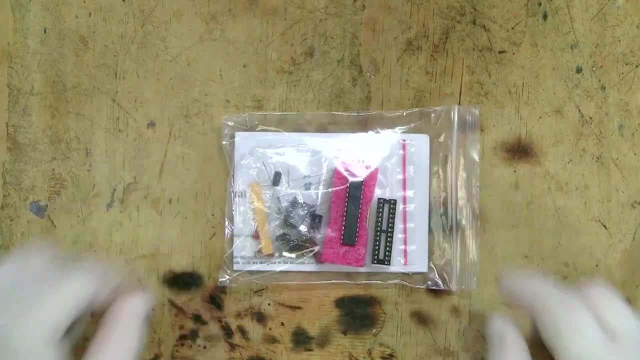 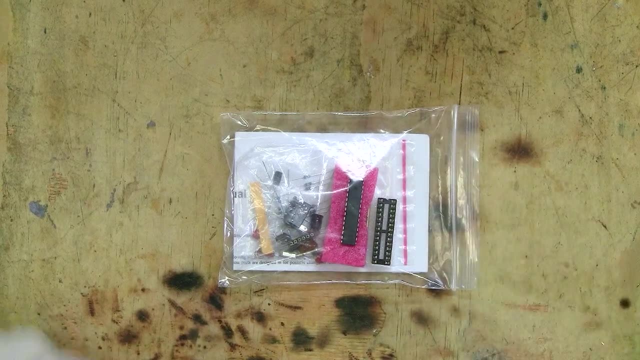 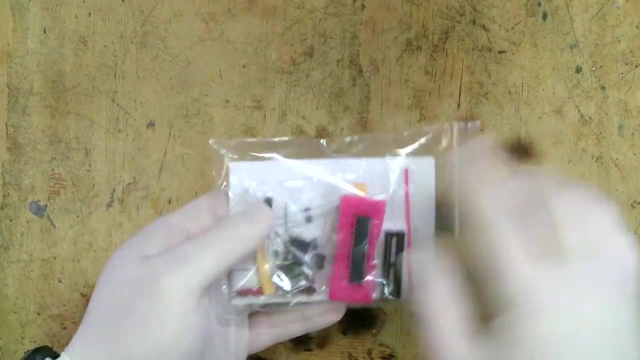 So let's get started. Here is the kit that we're going to be building today. I bought this one from Robot Gear here in Australia, but I will include links to other kit sellers in the description of this video. Let's have a look. We've got a printed circuit board. we've got some instructions.